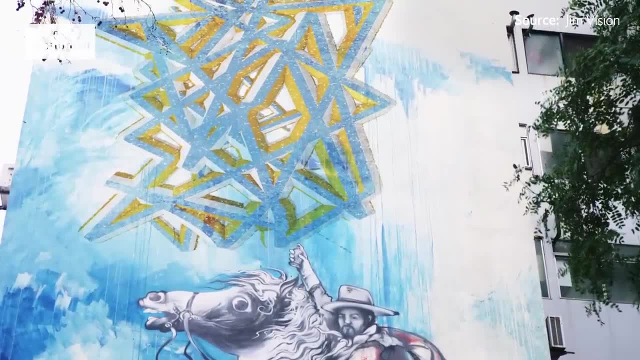 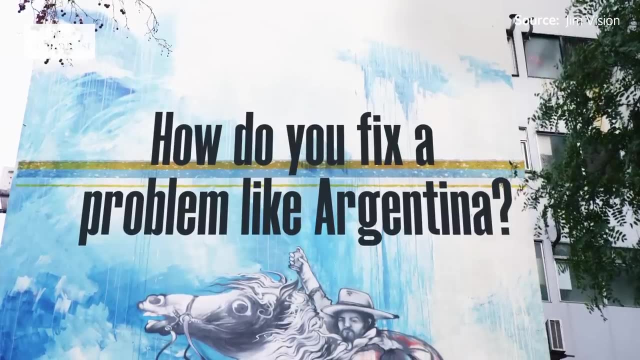 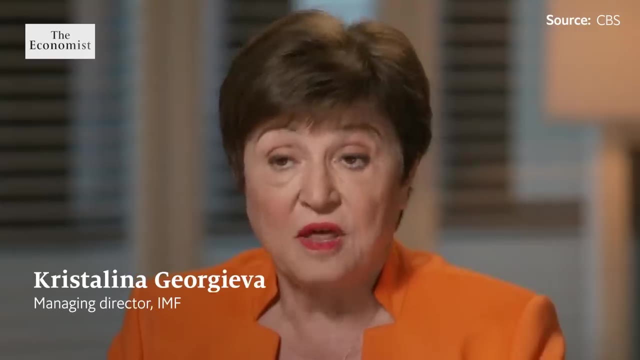 economic mismanagement over decades. without we see us going on on the front lines, Without big solutions, things could get much worse. Events of the past few years have been difficult for the world economy. This is going to be a tough year, tougher than the year we leave behind. 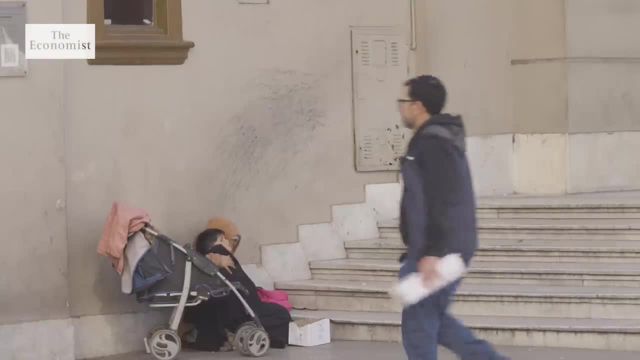 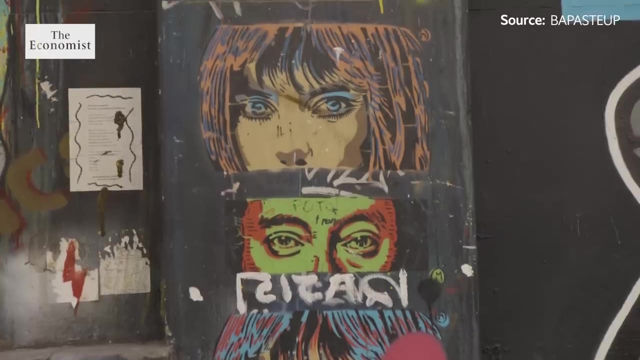 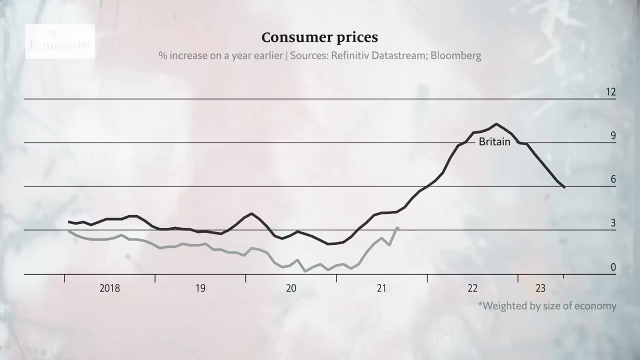 This financial storm hit when Argentina was already in peril To understand how bad it is for South America's second largest country. take a look at inflation. Countries like Britain have experienced annual price rises on par with the world average in high single digits. 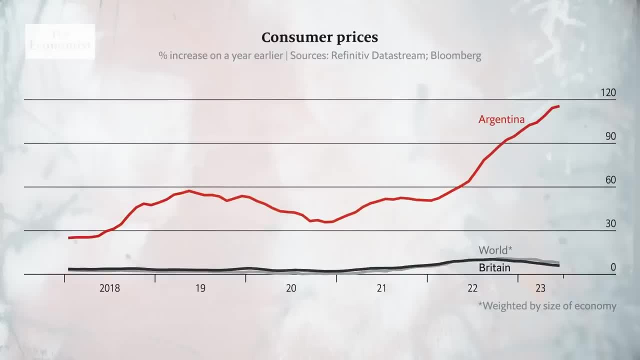 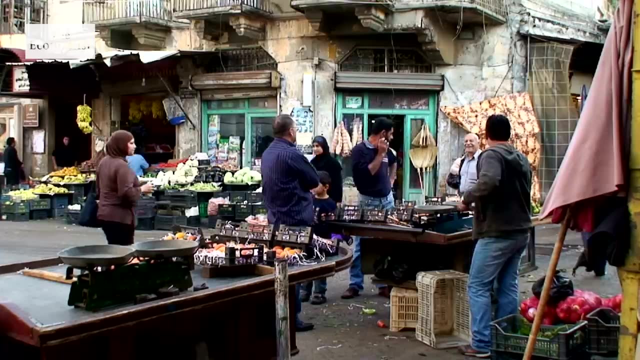 Argentina's inflation hasn't been that low in decades. The rate has been higher than 100% for almost all of 2023.. Right now, only Venezuela and Lebanon have higher rates. It's really hard to kind of just imagine what that's like. For some people they just can't make ends meet anymore. Inflation- this high forces many Argentines to get creative. Argentines save in dollars, because saving in local currency in a local bank has been a recipe for disasters. 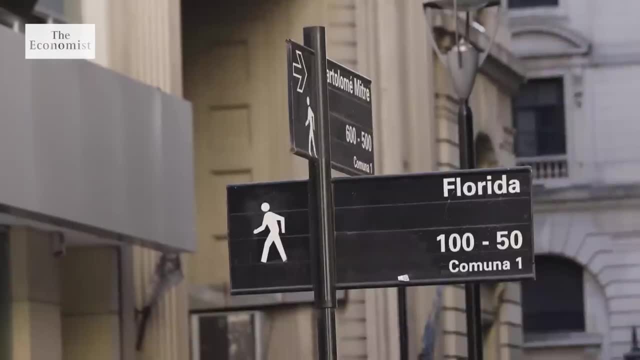 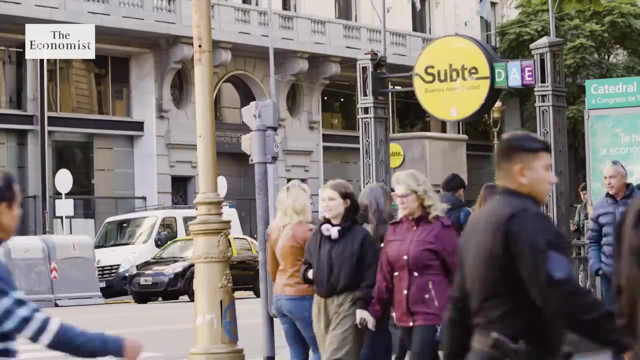 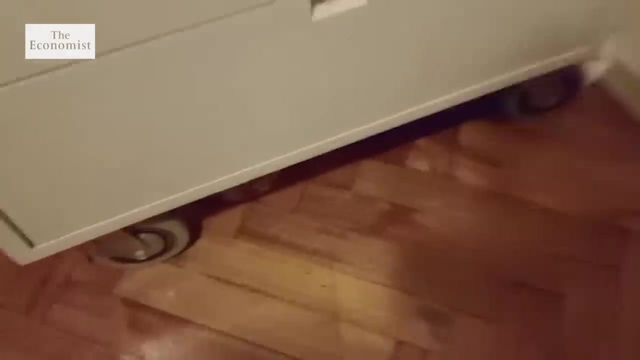 Even this isn't easy. Right now, Argentines can only legally buy $200 a month at the official exchange rate. That has created a vast black market for currency. Dealers line the streets of the city center While people hoard stashes of cash. 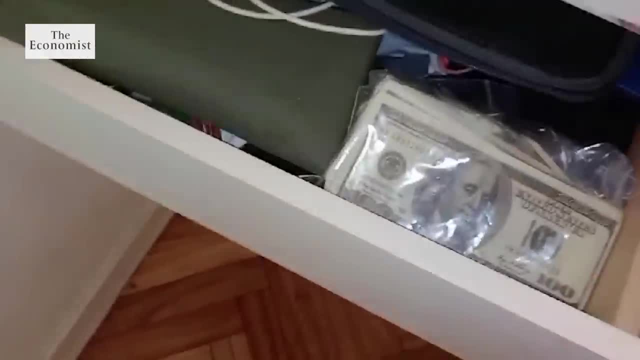 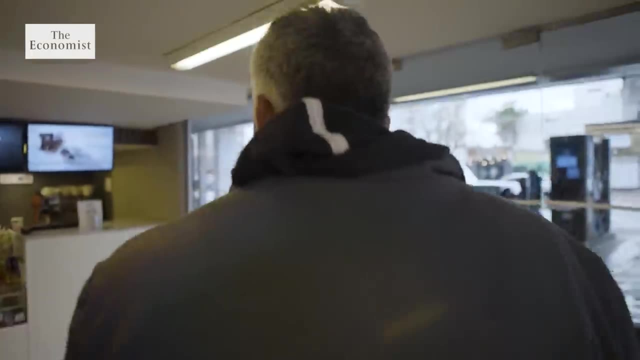 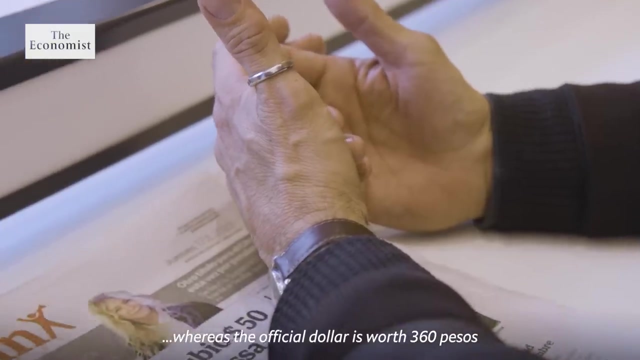 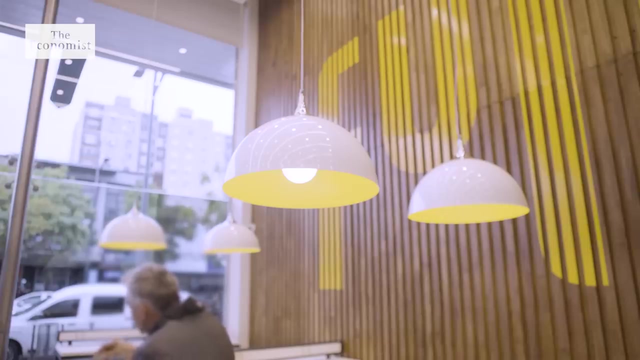 Cash at home, But buying dollars on the black market is more expensive than the official rate. Today the market has a dollar of 760 pesos against an official dollar of 360 pesos. The gap is enormous. El Flaco is one of a handful of bosses in Argentina's currency black market. 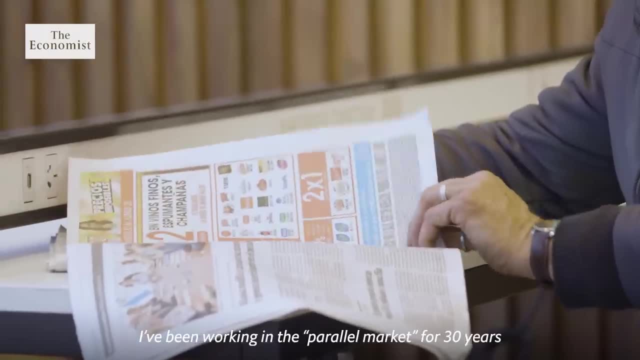 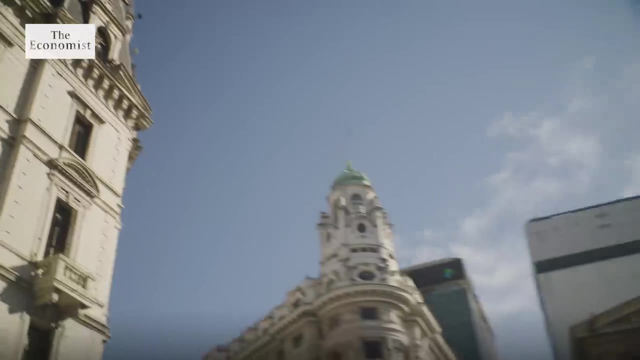 He's agreed to talk to us On condition of anonymity. I've been working in the parallel market for 30 years. There are 15 operators, no more than that. He claims the black market has tacit approval. In the stock market, absolutely everything is traded. 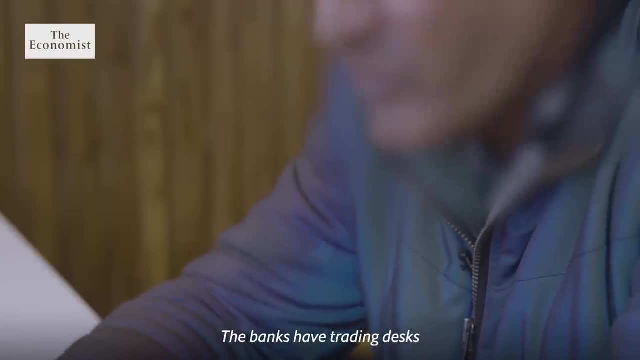 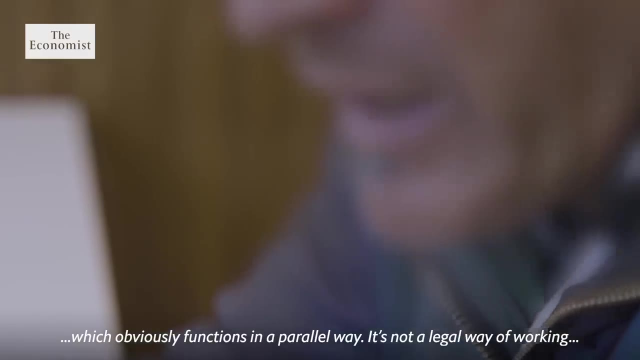 And it's also traded in the banks. The banks have tables of money In. that table of money is where the prices are formed. That obviously works in parallel. It's not a legal way of working, So let's say it's an illegal market. 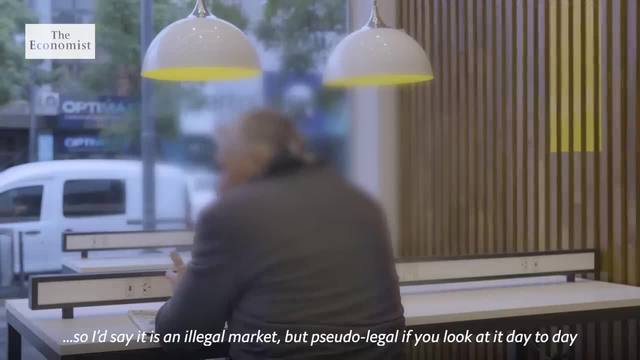 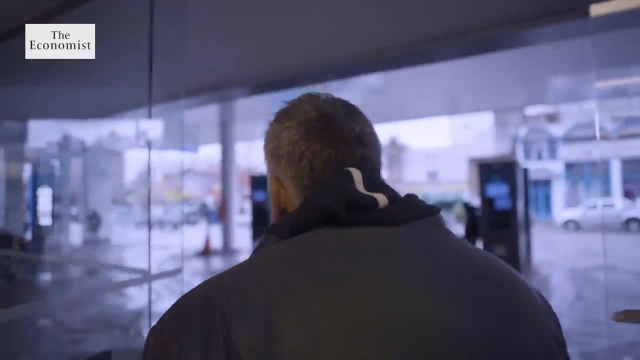 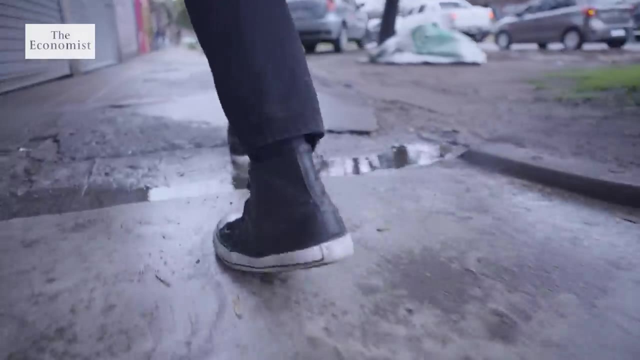 But it's legal, according to what you see every day. With a GDP of 630 billion US dollars, Argentina is one of the largest economies in South America, But this booming black market is a symptom of just how bad things are. 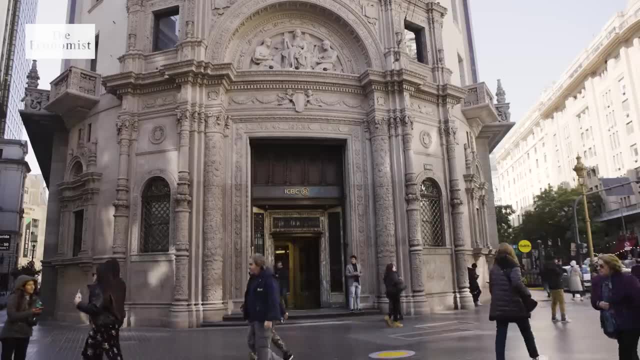 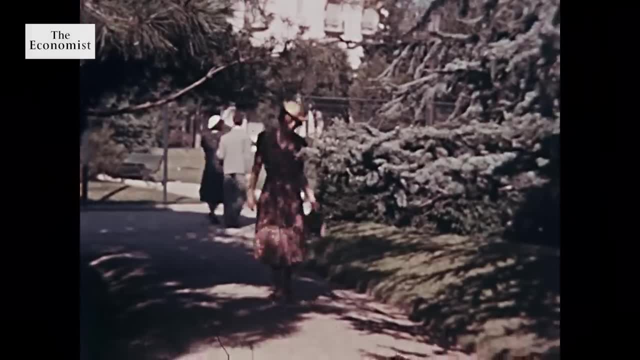 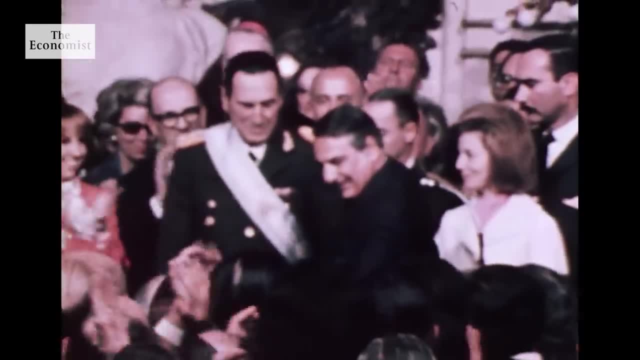 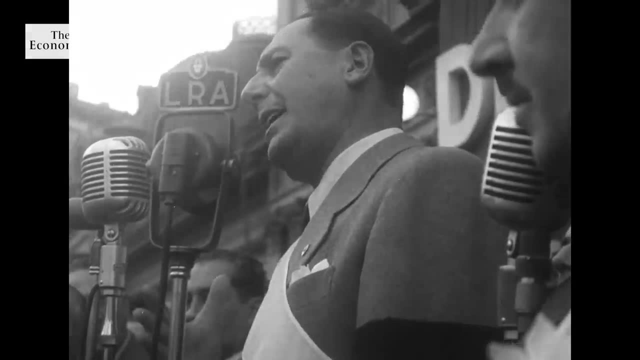 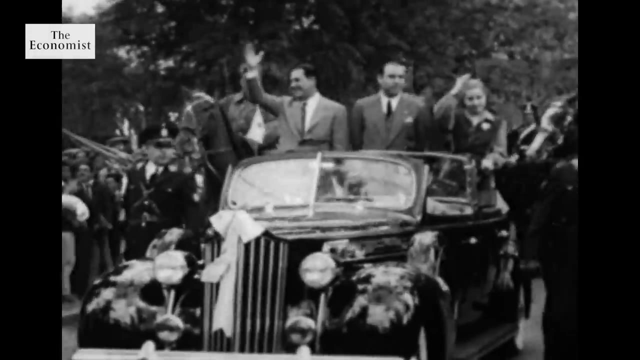 there are many reasons behind Argentina's decline, including the legacy of this man, Juan Domingo Perón, elected president in 1946.. He came to power after having been inspired by Mussolini's fascist Italy. Basically, what he took from fascism was a strong state. that's very intrusive. 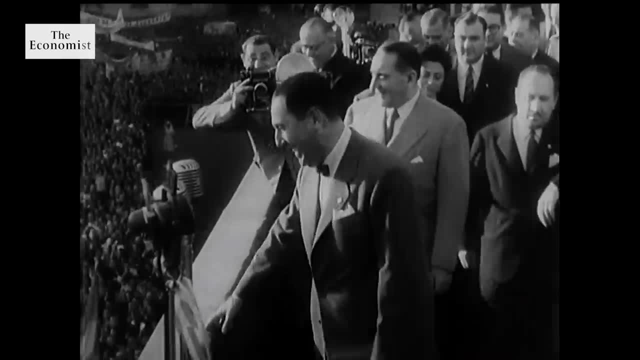 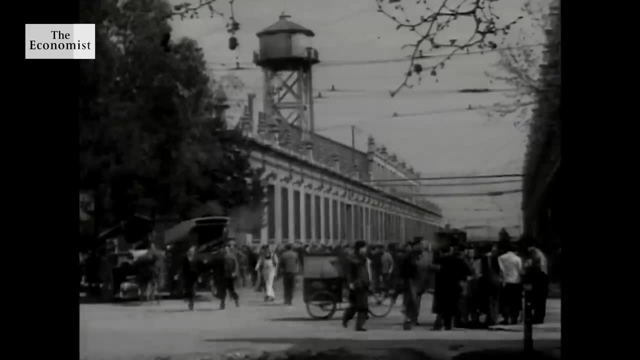 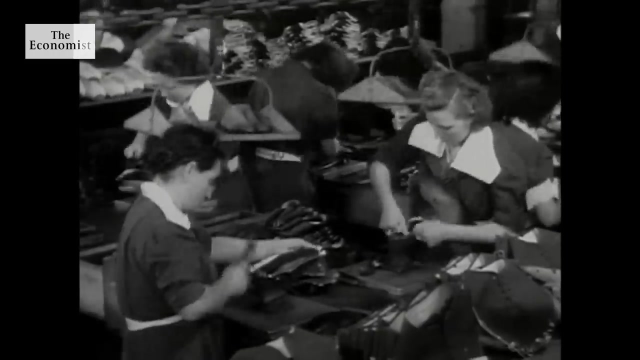 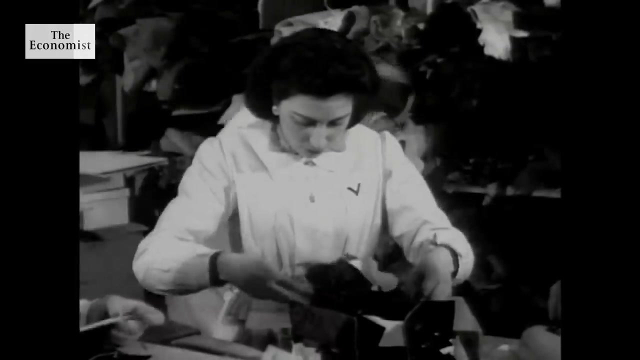 And a strong emphasis on nationalism. nationalism, And he combined that with also having a very strong labor movement. He introduced the eight-hour workday, increased wages for the poor and created vast, expensive welfare schemes. He also embraced economic isolationism. The emphasis on national sovereignty led to kind of the coddling of workers by 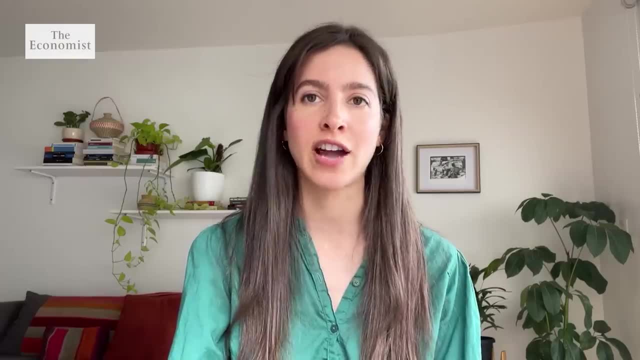 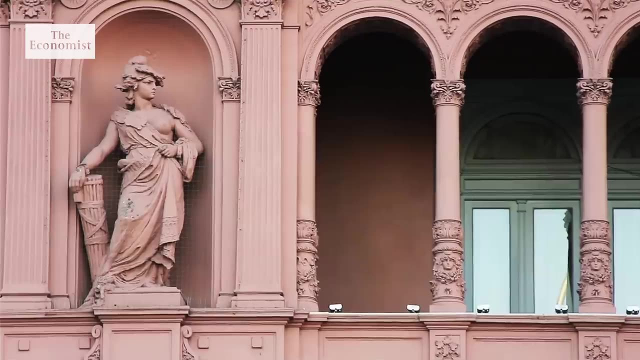 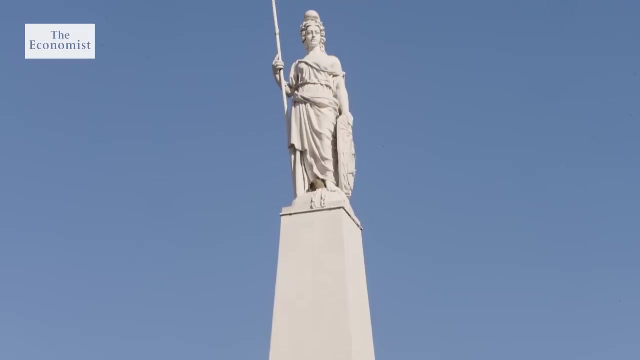 protecting them from foreign competition that has shut itself off from international trade. Today, Argentine politics is still dominated by his legacy. Peronists have been in power for 16 of the past 20 years. One of the issues with Peronism is they haven't evolved with globalization and 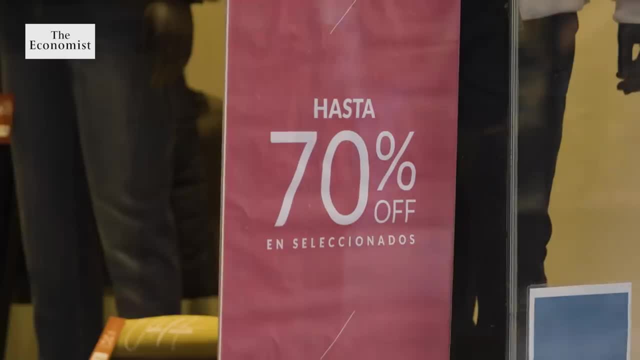 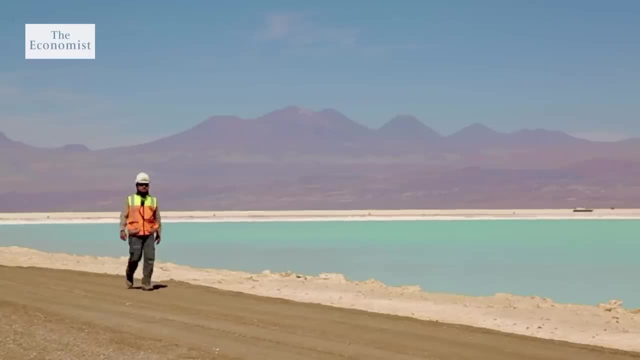 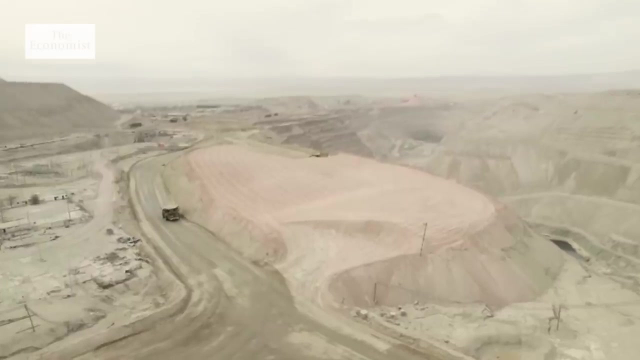 with the world. Argentina's exports have shrunk as a percentage of global exports year after year In the mining sector. Argentina has one of the largest reserves of lithium and also it's very rich in copper- just to think that Chile is the biggest copper exporter in the world- and 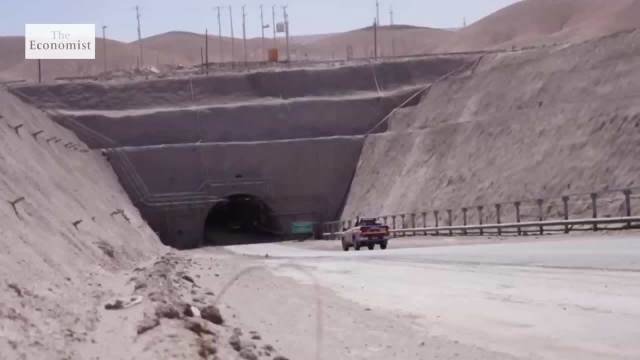 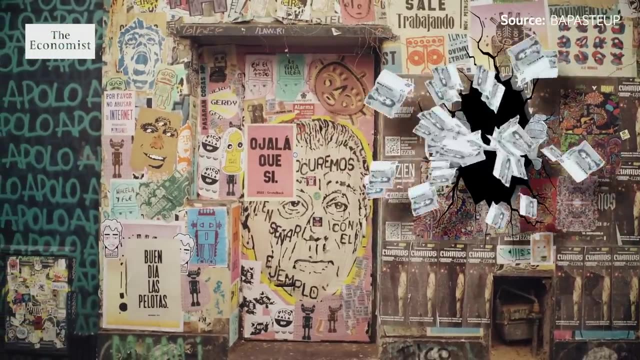 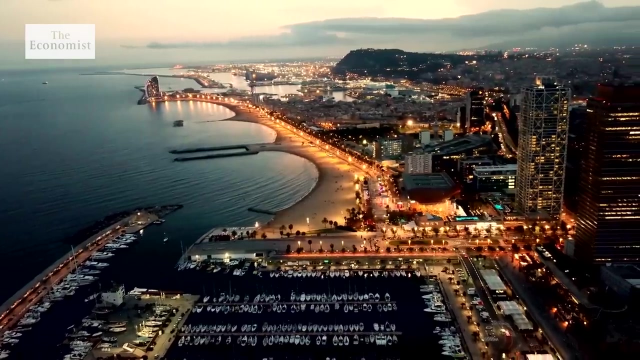 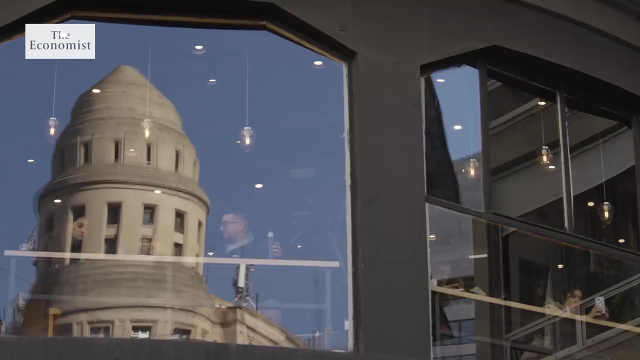 Argentina produces zero copper and we share the same mountains. As well as remaining isolated from the world economy, the government also still hugely overspends on things like price subsidies. The average European spends around $40 a month. on electricity, The average Argentine spends $5, eight times less. 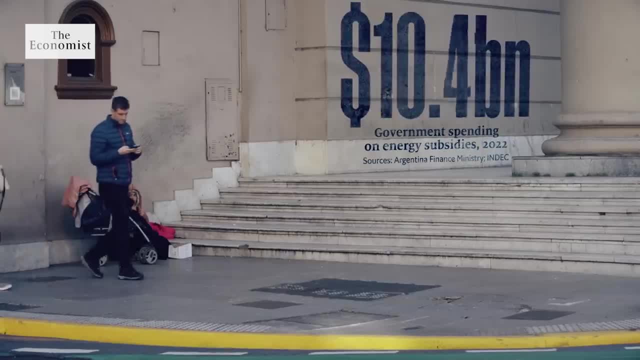 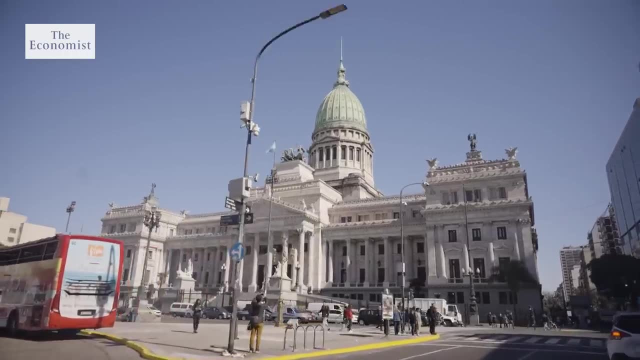 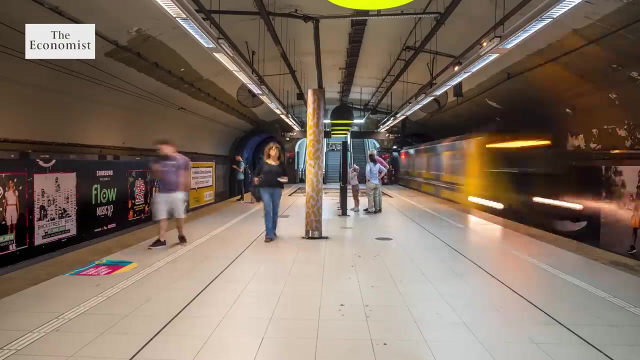 In 2022 alone, this cost the government $12.5bn- around 2% of Argentina's GDP. But government largesse goes beyond welfare. Of the 13 million people in formal employment in Argentina, over a third of them are employed by the state itself. A lot of spending goes on paying salaries and pensions. You actually want it to go on things like investment, technology, infrastructure, helping the poor, rather than paying public wages. All of this points to the main issue in Argentina's economy. Argentina has been running a fiscal deficit for the last 13 years. If you're in a difficult time for 13 years in a row, well, you have a big problem. Policies to counteract this deficit, like printing money, only make things worse. 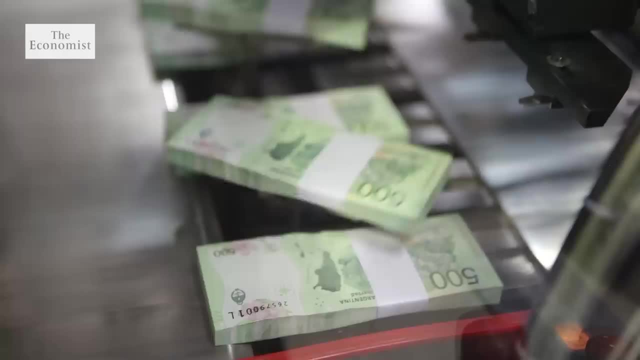 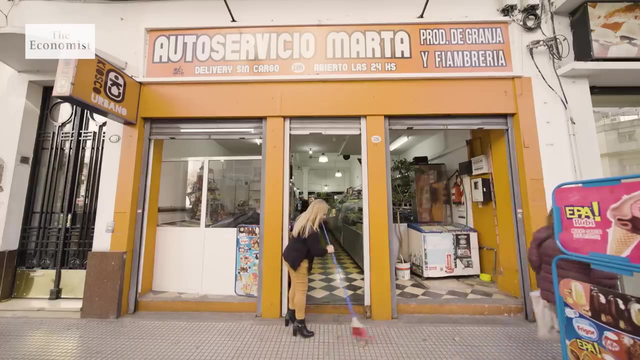 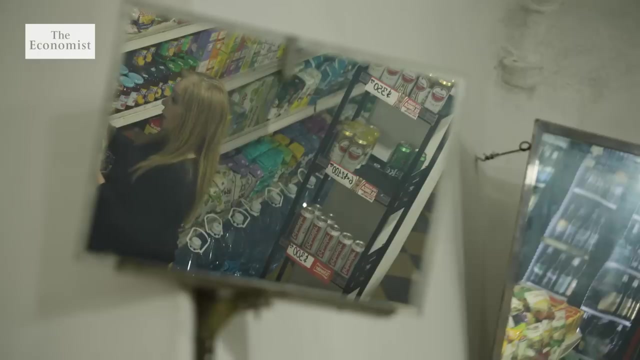 Governments have become dependent on the central bank printing money to basically finance spending, And the more money you print, the worse inflation gets. Local shopkeeper Marta Valdez feels the direct impact of more money being pumped into the system. Here we have 1,000, 2,000, 3,000, 4,000 pesos with all this. 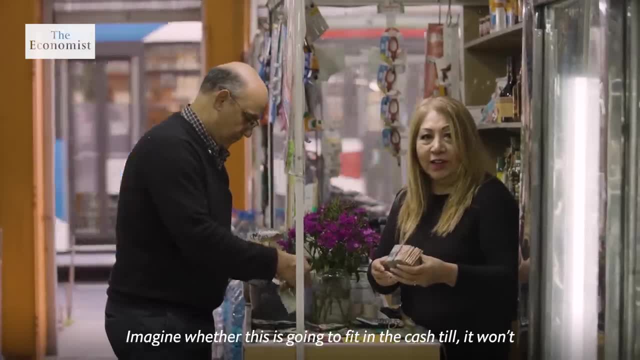 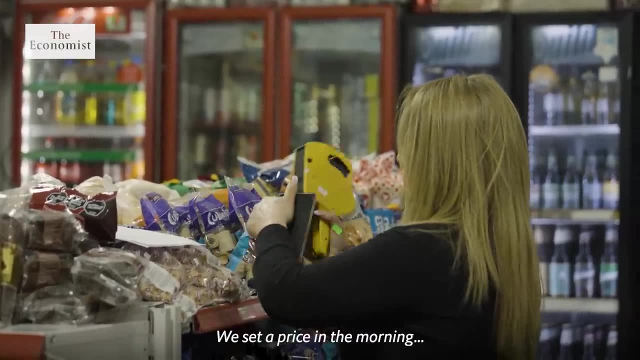 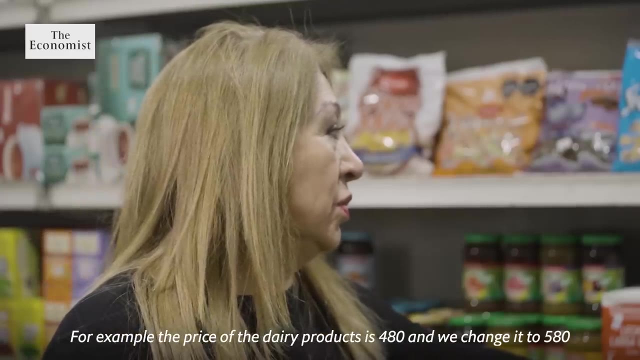 Look, if this goes into the cash register, it won't. If it goes into circulation can mean it's worth less. If we set a price in the morning, maybe in the afternoon we'll set another price. For example, the price of dairy products is from 480 to 580. 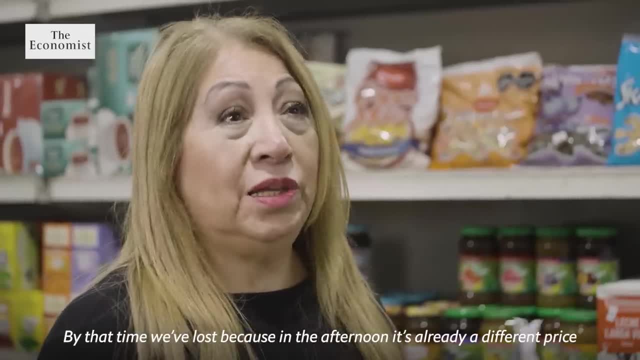 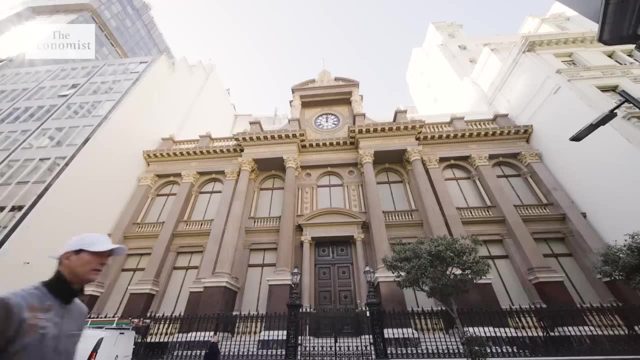 In that period we lost, because in the afternoon it's a different price. You work for nothing because you don't earn anything. But printing money is only one way the government tries to make money. Printing money is only one way the government tries to fund its spending. 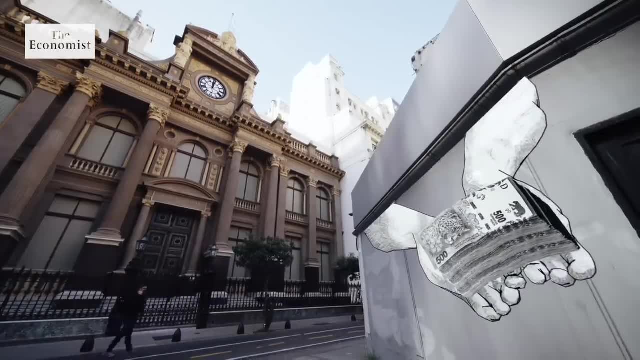 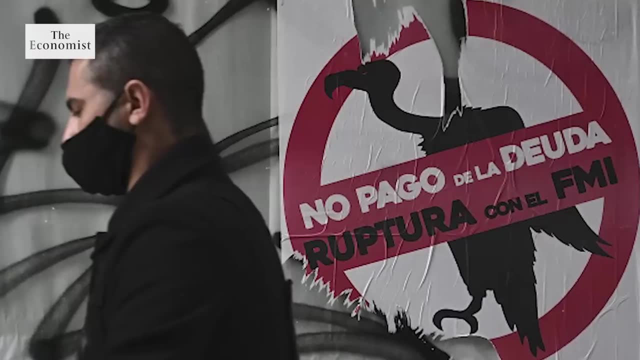 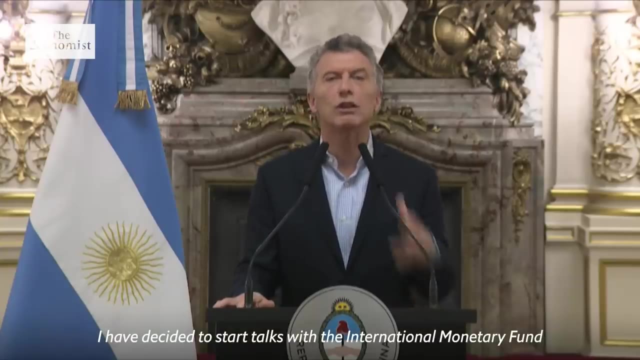 Another is borrowing. So Argentina has borrowed a lot of money, but it has also defaulted so many times that people don't want to lend it money anymore. Despite the risks, there is one institution that continues to lend. I've decided to start conversations with the International Monetary Fund. 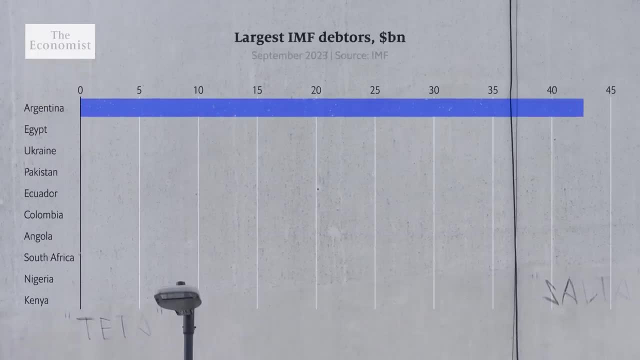 Today, Argentina's debt to the IMF is more than double that of Egypt, the second highest borrower. All told, Argentina holds almost a third of all of the IMF's total lending, One of the criticisms that most economists have posed to the IMF. is that the conditionality that they put to Argentina was so, so light. They didn't need to stabilize the economy, they didn't need to do any homework and they received money. I think that was another missed opportunity for Argentina. Borrowing and printing money are not unusual tactics for governments. 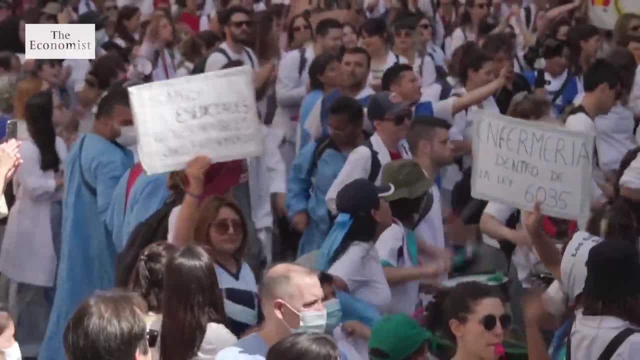 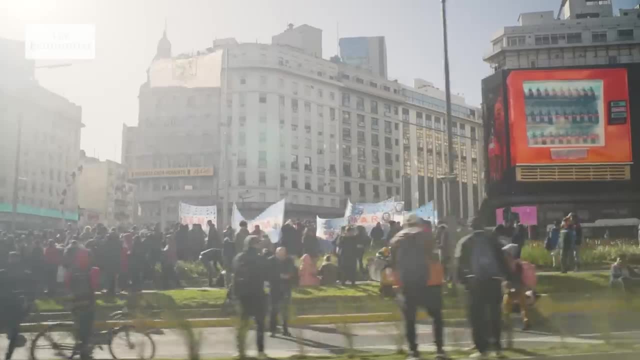 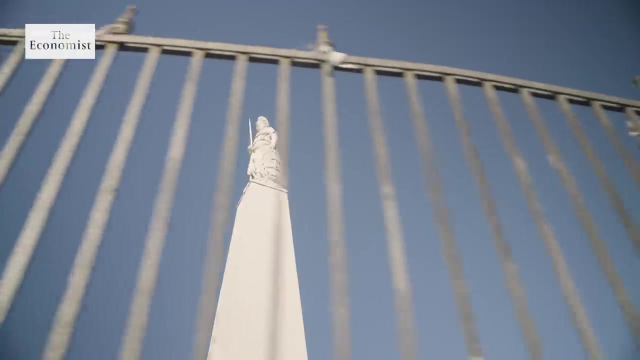 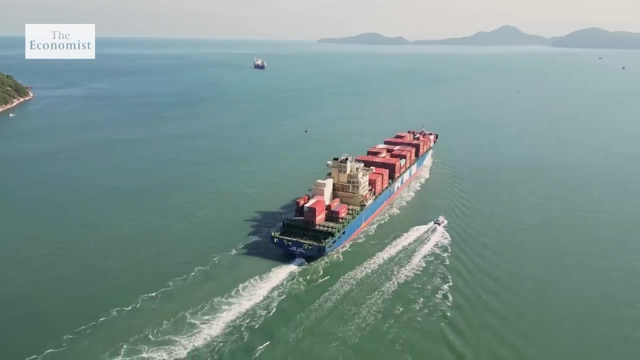 but the extent that Argentina's government does both is extreme and damaging, In part because loans from the IMF need to be repaid in foreign currency, And one tactic Argentina employs to get that foreign currency only complicates things more: Trade restrictions. Soybeans are one of the country's biggest exports. The soybean producer in Argentina. they face an export tax of 33%. If a ton of soybean costs, say, $500, I receive $500 minus 33%, Leaving the farmer with $335. They then have to exchange these dollars for pesos at the official exchange rate. 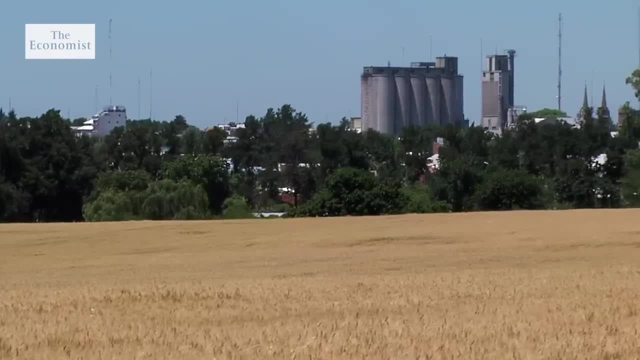 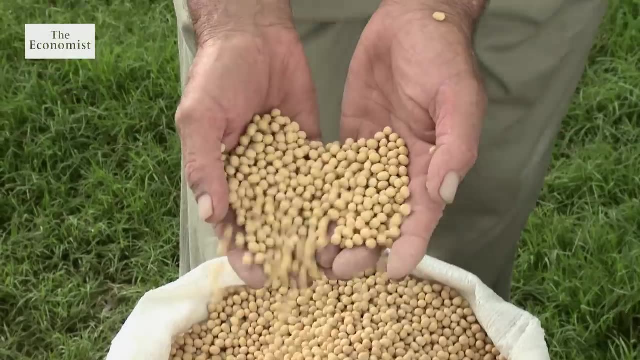 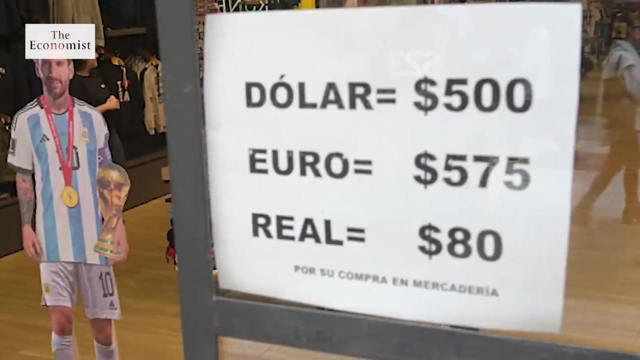 When the dollar rate is bad, farmers have to make harsh decisions. The incentive is to keep your soybeans in your silos until the exchange rate changes. If everybody does that, the supply of dollars in the economy is scarce. So the government invented something that we call the soybean dollar. 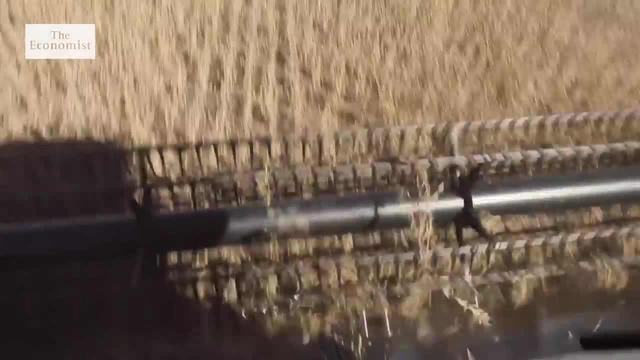 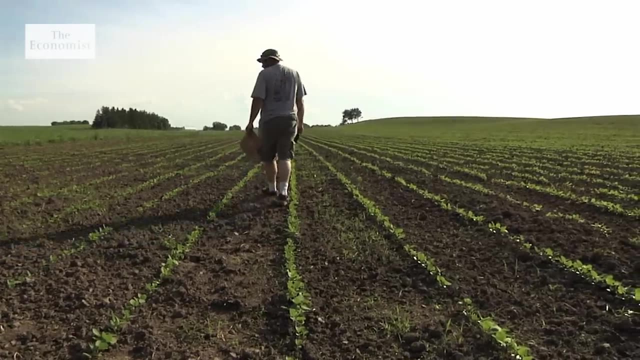 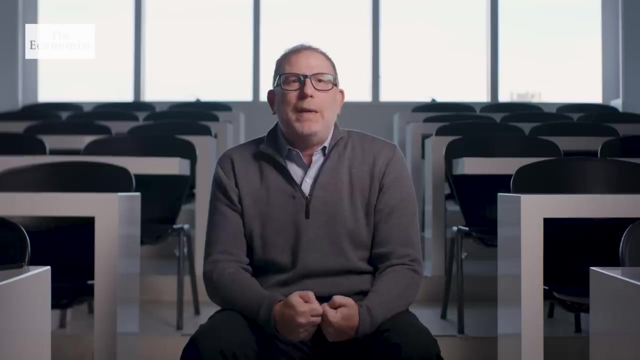 The soya dollar is a slightly better exchange rate, specifically for profits on soya exports. But it's not the only market with confusing rules. If you want to organise a concert in Argentina and bring a British singer, you have to pay the official dollar and then an extra tax. 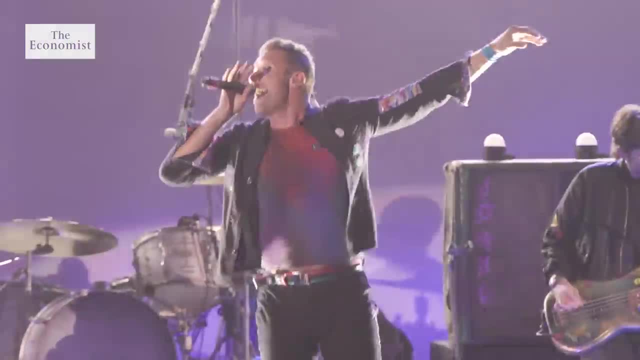 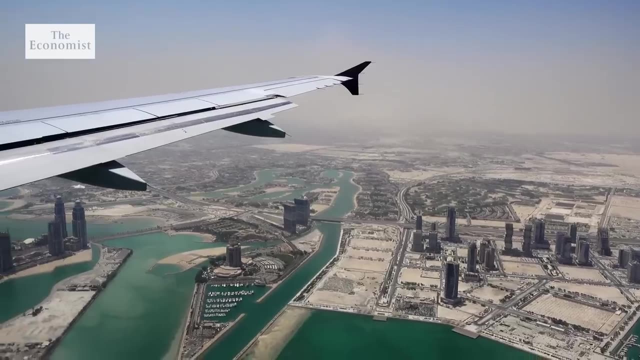 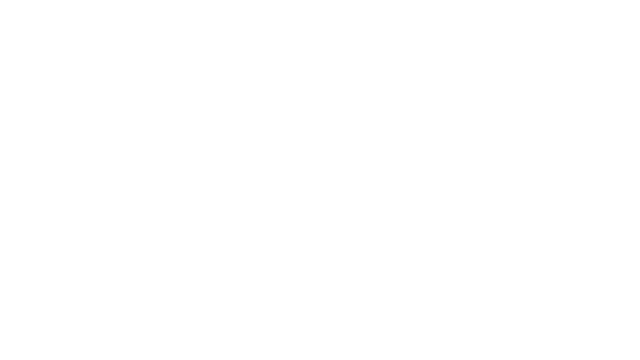 We call it the dollar cold play. If you want to travel abroad, you use your Argentine credit card and you pay the official dollar plus taxes, And we call that the dollar Qatar. This idea of having 10,, 15,, 20 different prices for the same thing. 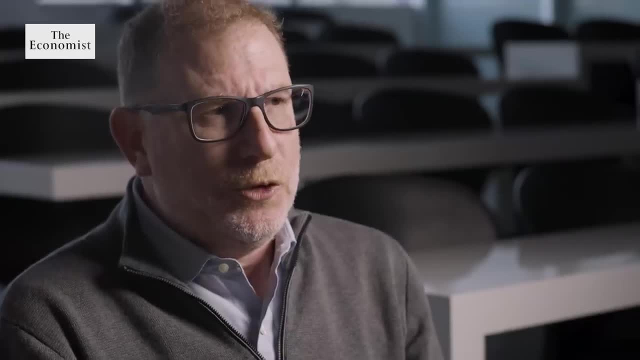 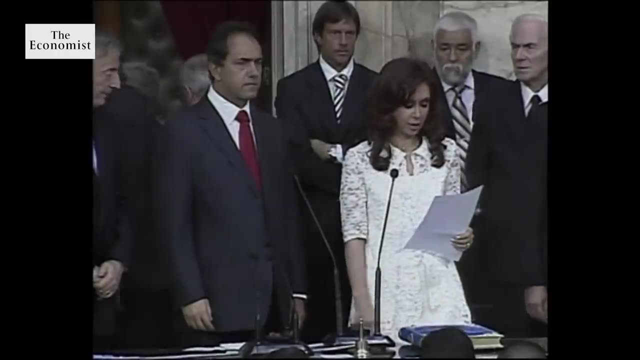 doesn't make any sense. That's a distortion. With a set of distortions, it's impossible that Argentina grows. Over the years, different presidents have proposed different solutions to the economic conundrum, but the outcome tends to be the same. 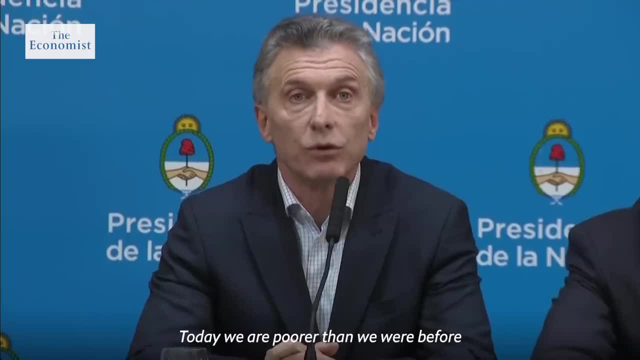 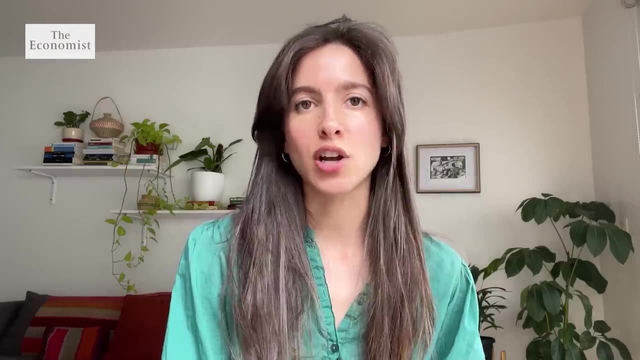 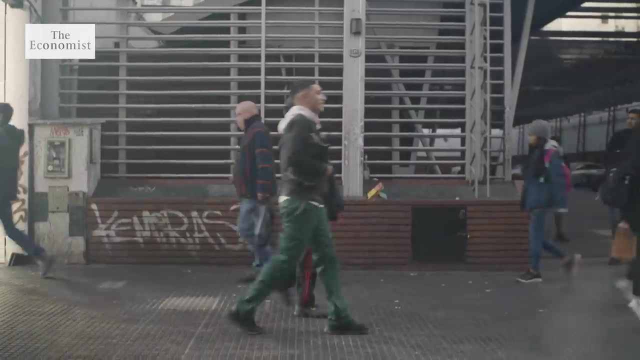 More debt and more inflation. Today we're poorer than ever. It's really really hard to fix Argentina's economy, and that's because many of the things that we've talked about are linked. Everybody agrees the government needs to spend less. One way to do that is by reducing subsidies. But if you do that you're going to push up inflation. Everyone knows the currency needs to be devalued and if you devalue the currency, that will also push up inflation. So it's really hard because tackling one part of the puzzle.